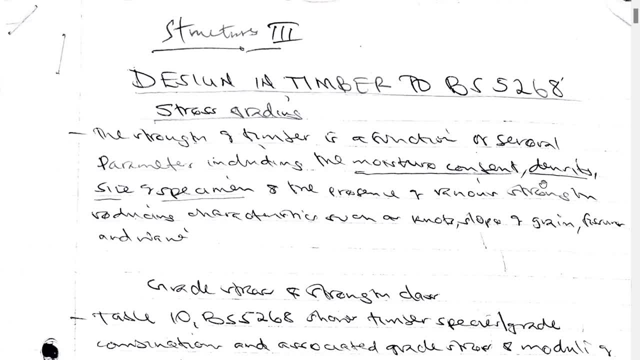 is inversely proportional to the moisture content. Now, when you talk about density, you find that the strength of the timber relates positively with the density. When the timber has a high density, it has a high strength. Now we look at the size of specimen Automatically when 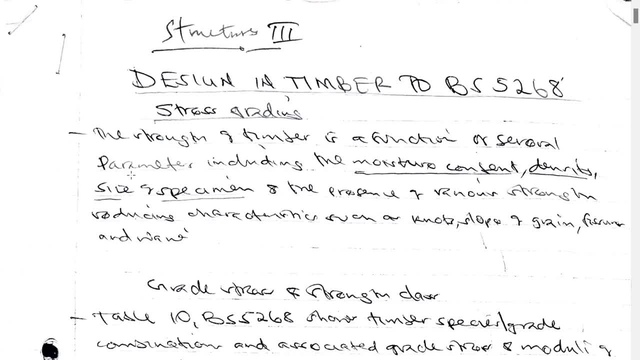 we have a large piece of timber, we expect it to be more strong compared to a small piece of timber. So when we look at the size of specimen, we expect it to be more strong compared to a small piece of timber. Another one is presence of various strength reducing. Now, when you talk about 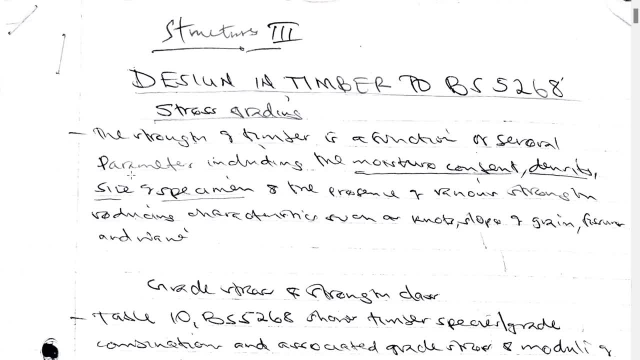 knots. knots can be like rods in our timber. Then slope of grain. the slope should be uniform for the timber to be of good strength. Then fissures means some unfilled holes or spaces within the timber section. They reduce the strength. Then we have when, when or when is where now the timber? 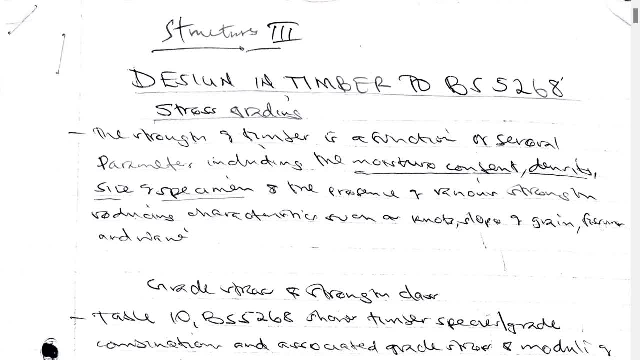 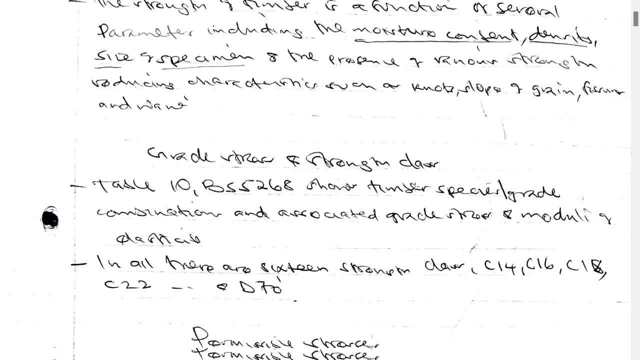 if the section will be fully rectangular, you find like some parts of it have been removed, have been chopped off. So then we reduce the strength of timber. Now let's go to stress grade, stress and strength class. So table 10 of BS 5268 shows: 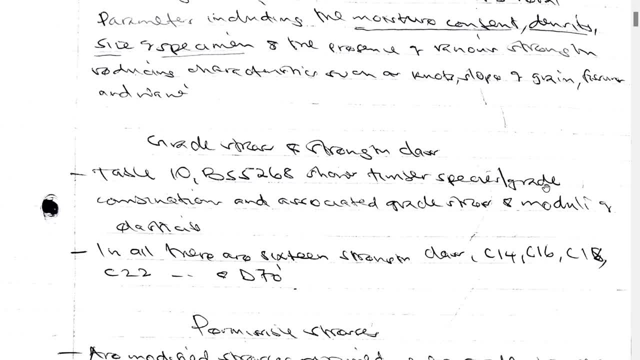 timber species, or what we call grade combination, and associated grade stress and moduli of elasticity. Now what we mean is that this table 10 of BS 5268, you will find like we have timber classes like class C14. It gives you the bending stress, the shear stress. 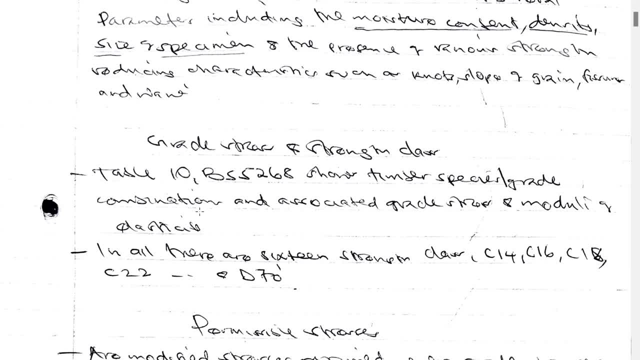 the compression stress. You give it the modulus of elasticity, So you move along a row and rotate the properties of each of the timber classes. So in all there are 16 strength classes. So the grade stress or strength class, we have 16 of them And the most common one we have class C14,. 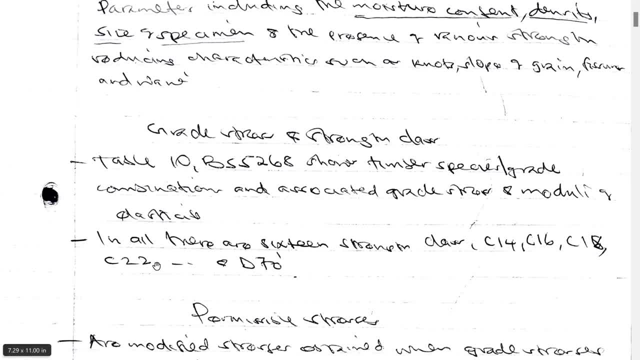 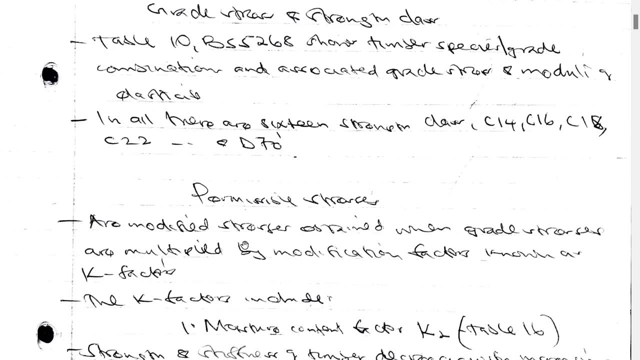 class C16, class C18, class C22, up to class D70.. Now, from there, let's look at what we call permissible stresses. So when we talk about permissible stresses in simple term, we mean the amount of stress this timber section can withstand without failure, Like we mean. 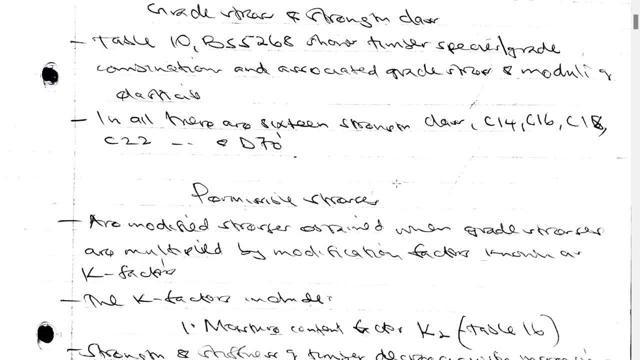 if permissible stress of a timber is 20 nm2,, if you apply a load of 21 nm2, the timber section is likely to fail because the stress will be more than what it can accommodate. permissible stresses are modified stresses obtained when grade stresses are multiplied by modification factors. 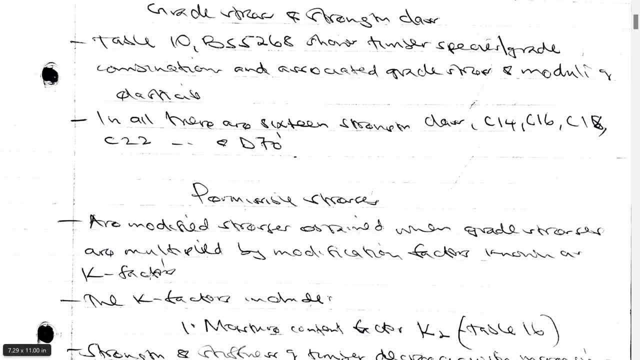 known as the K factors. Now, when we talk about grade stresses, grade stresses is the value obtained from table 10 of BS 5268.. So the value obtained from table 10 of BS 5268, when you multiply by the K factors. 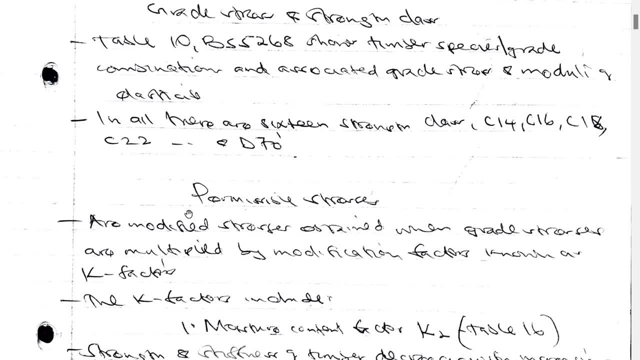 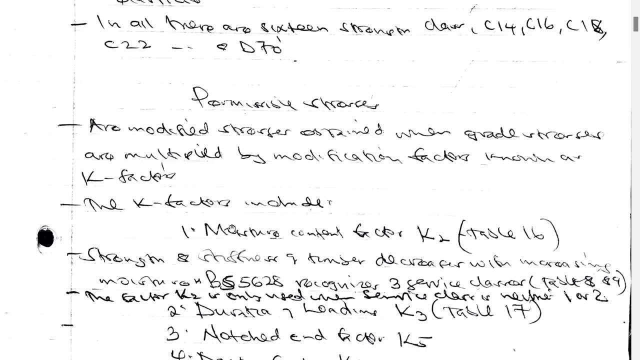 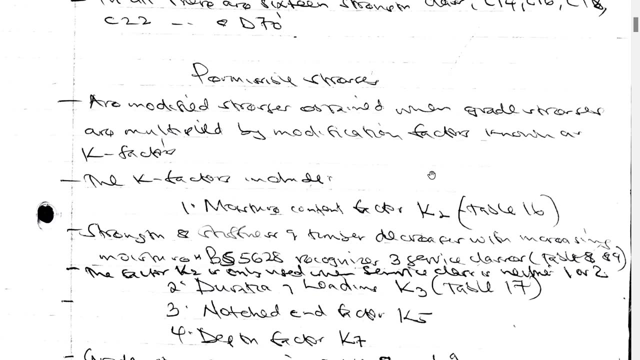 the result you get are called permissible stresses, So the K factors include. so we have these K factors come in different form. We have the moisture content factor, So the moisture content factor is given as a K2.. So it's a K factor, but K subscript two. 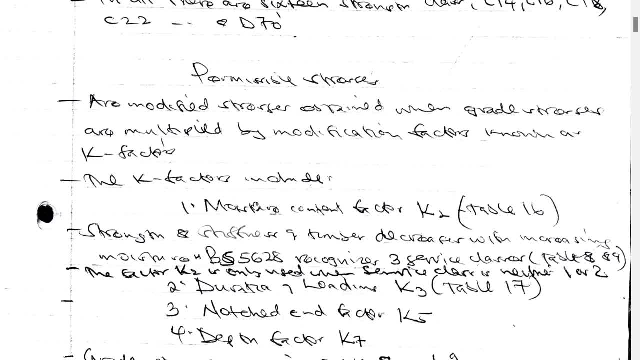 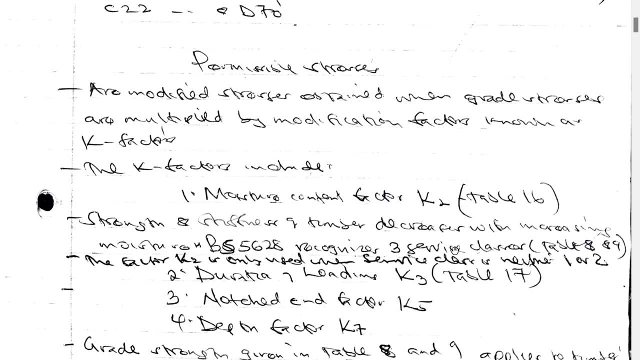 Now it is in table 16 of BS 5268.. So you find that, as I said earlier, strength and stiffness of timber decreases with increasing moisture content, Like where the moisture content is high in a timber section, its strength will be low. 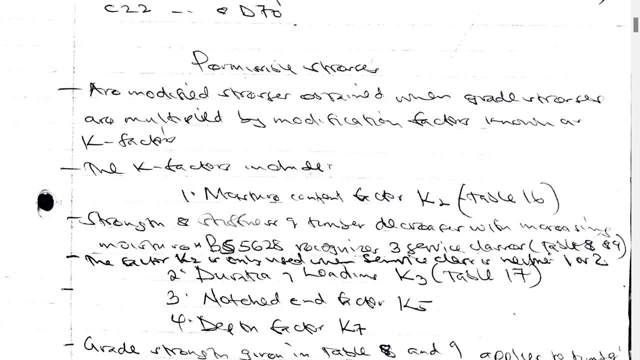 So from BS 5268, you find that we have three service classes, which can be seen in table eight and nine. So we have service class one, service class two and service class three. Now for you to apply the factor. 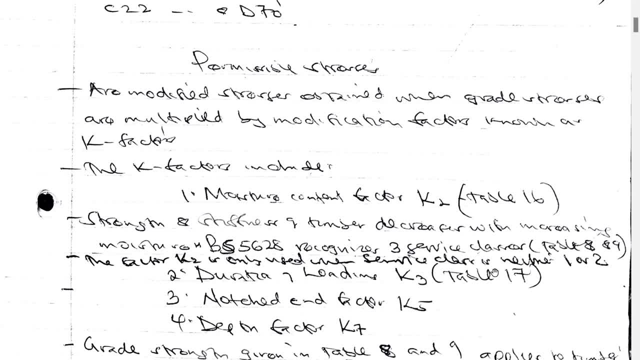 K2, the service class of the timber should only be three, but for service class one and two we don't use K2.. So to find more about what is service class one and two, you can refer to the notes on moisture content factor K2.. 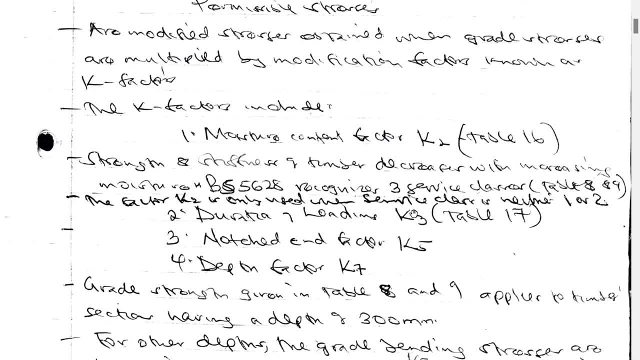 Then another K factor is duration of loading, which is given by K3.. So the duration of loading, K3, we have three cases: We have short-term, medium-term and long-term loading. So you can obtain them in table 17 of BS 5268.. 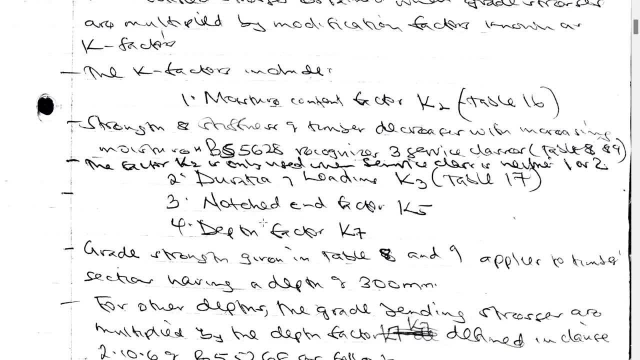 Then we have notched end factor. Now, notched end factor, it means our timber sections at their end they are connected in form of notches, grooves and notches, So it's factor K5.. Then you have depth factor. 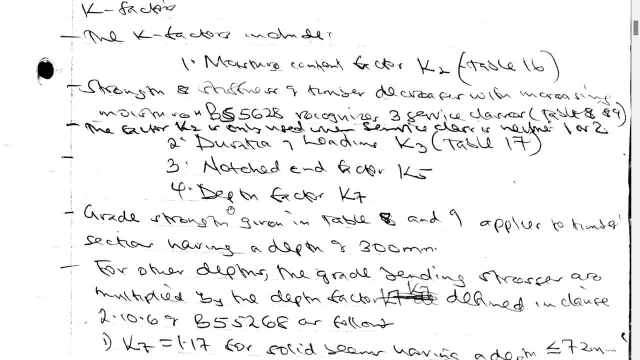 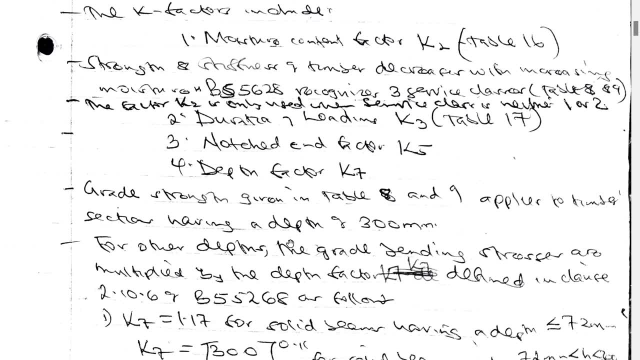 which is K7. And, as I said, grade strength given in table 8 and 9 apply to timber section having a depth of 300 millimeters. So these K7 values from table 8 and 9 are only for timber sections. 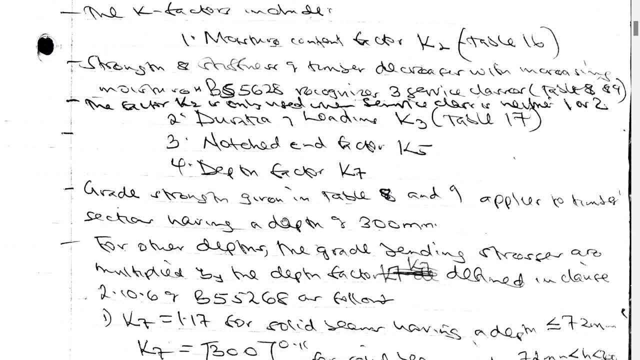 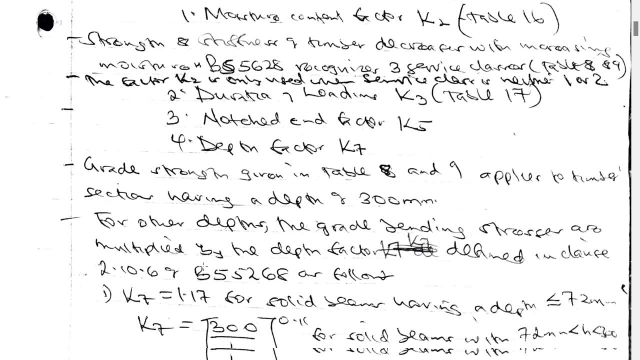 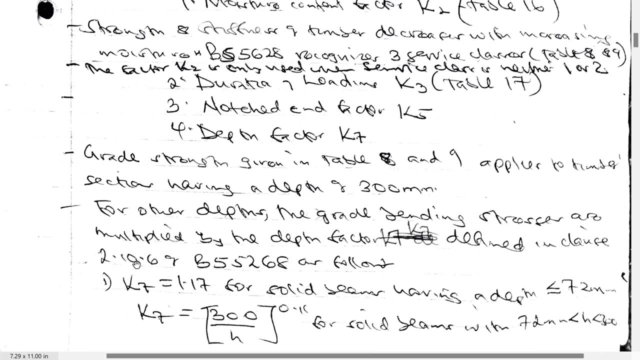 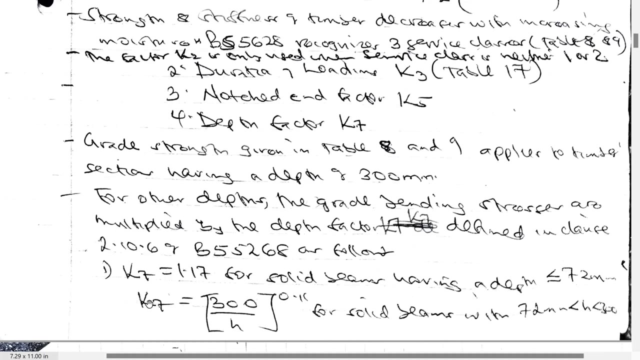 which have a depth of 300 millimeters. So for other depth, the grade bending stresses are multiplied by the depth factor K7, defined in clause 2.10.6 of BS 5268 as follows: Now remember, the K7 value in the table is for a depth of 300.. 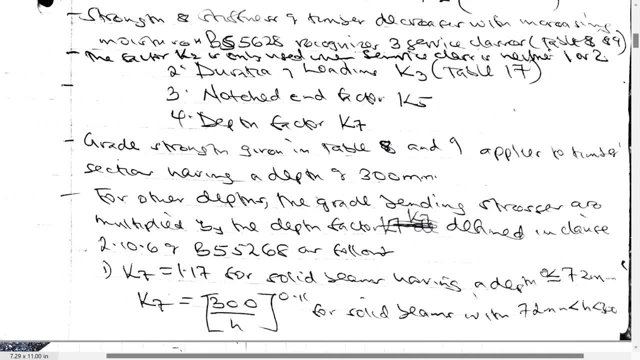 But now, if my section depth lies below or equal to 72,, my K7 is equivalent to 1.17.. It will be a constant. But if my depth of the section lies between 72 and 300, then K7 will be equal to 300 in millimeter. 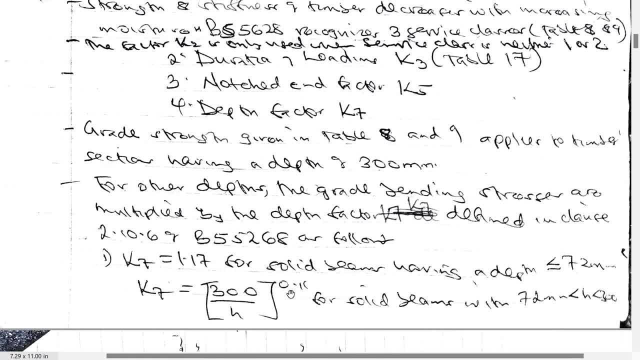 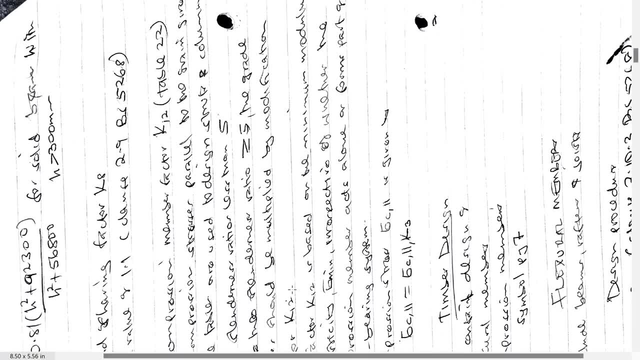 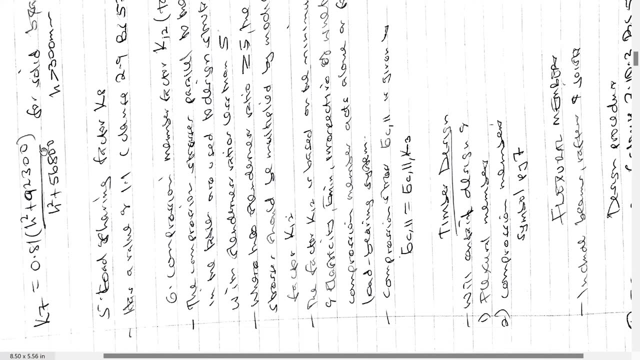 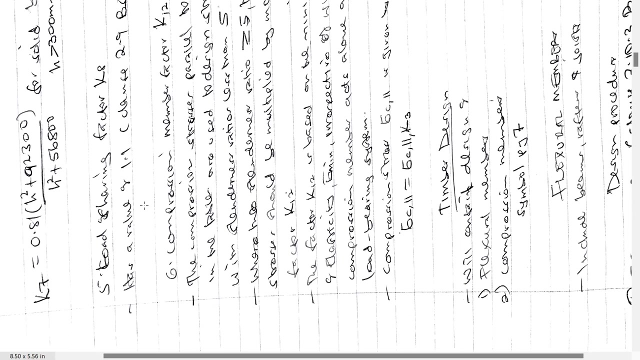 divided by depth in millimeter, or that power 0.11.. And then you find that we have some cases. we have some cases whereby maybe your section's depth is more than 300 millimeters And then, in such a case, our depth factor K7 would be 0.8 into H squared plus 92,300,, which is a constant, divided by H squared plus 56,800,, which is also a constant. 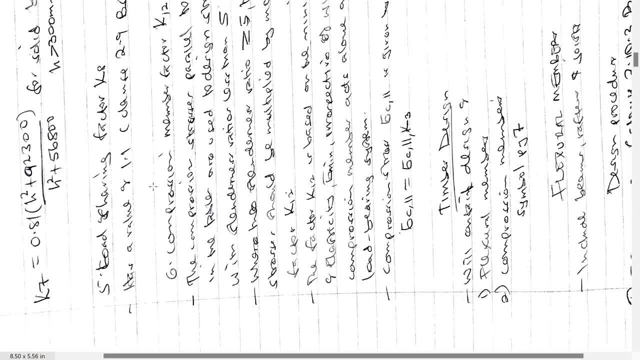 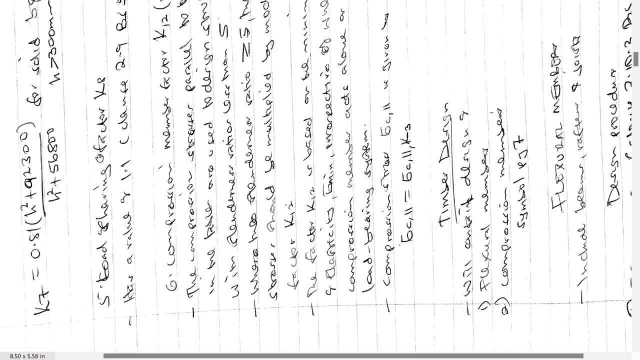 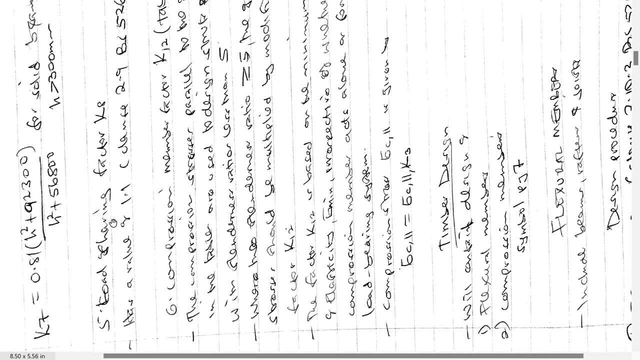 Then we have another K factor called load sharing factor K8. So this load sharing factor K8 has a value of 1.1.. It's found in clause 2.9 of 52.68.. Now you find that for me to use the load sharing factor it means you must have a system of joists. 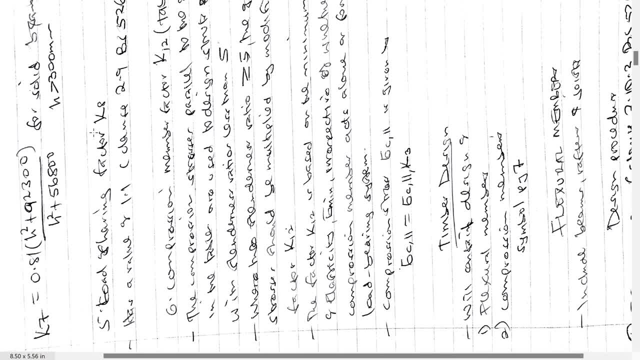 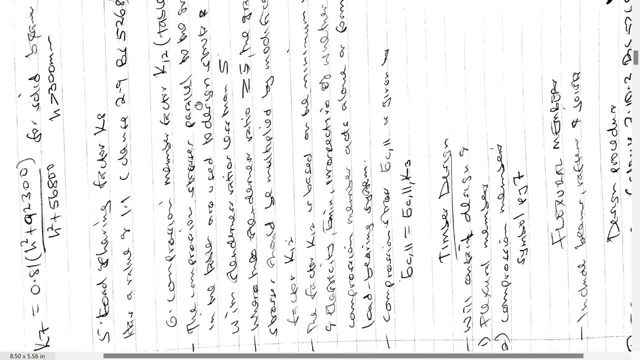 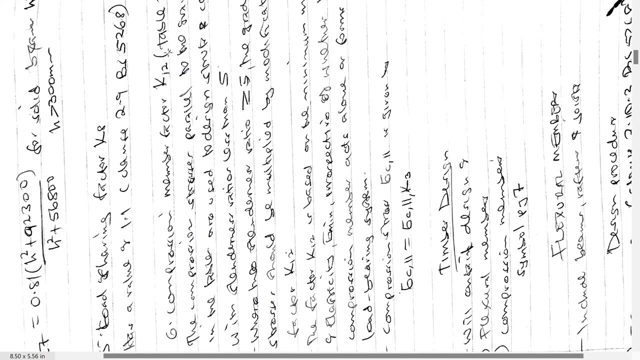 Timber joists means secondary beams which are sharing the load and transferring the same load to the main beams. Another K factor: we have compression member factor K12, table 22.. So compression member factor K12 only applies to the columns and steps, Because columns and struts are compression members, while beam and slabs are flexural members. 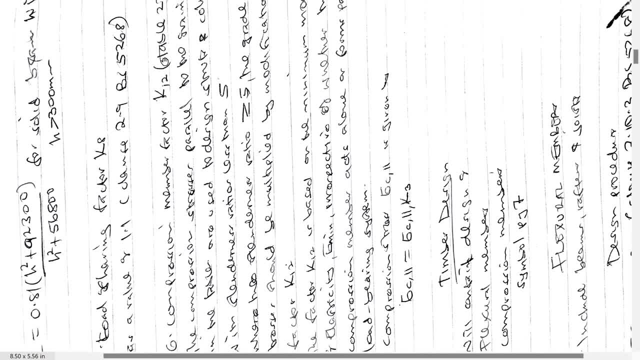 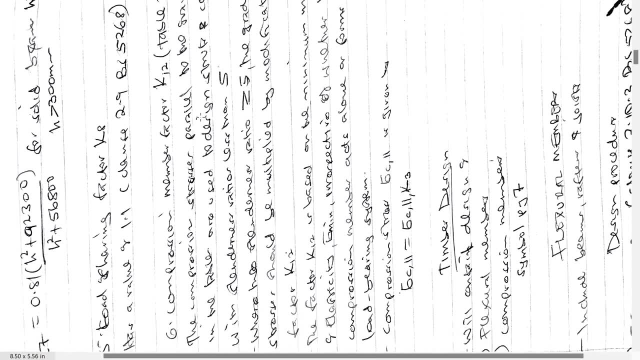 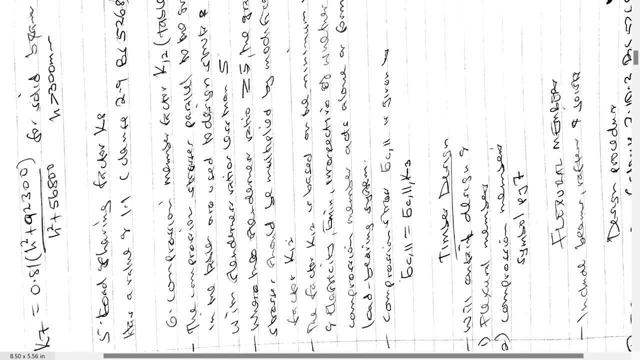 So compression factor K12 can be obtained from table 22.. So the compression stresses parallel to the grain given in the table are used to design struts and columns with slenderness ratio less than 5. So where the slenderness ratio is, 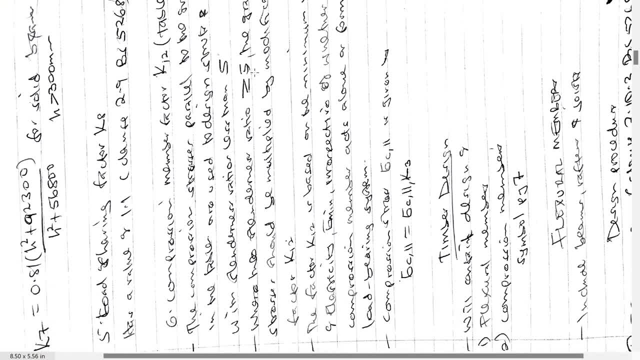 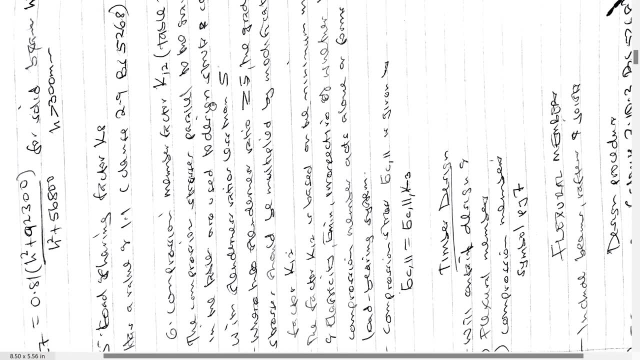 Equally greater than 5.. The grade stress should be multiplied by modification factor K12.. Now from that table you find that the table 8 and 9, where we have the grade stresses. those values are given if the slenderness ratio of a compression member are below 5.. 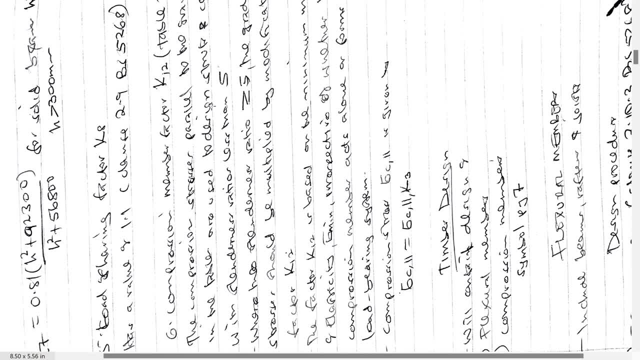 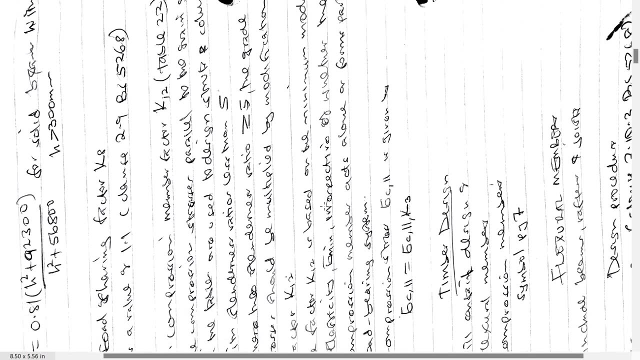 But if you calculate and find that slenderness ratio is equal or greater than 5, we have now to modify the grade stress. So we have to modify the grade stress using the factor K12.. So the factor K12 is based on the minimum modulus of elasticity. 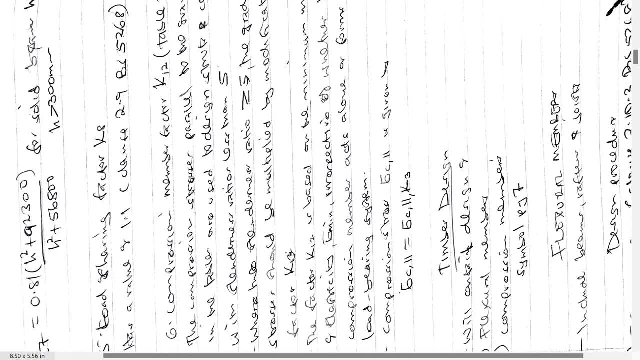 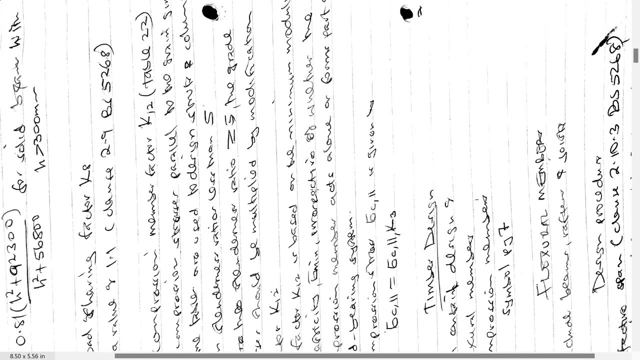 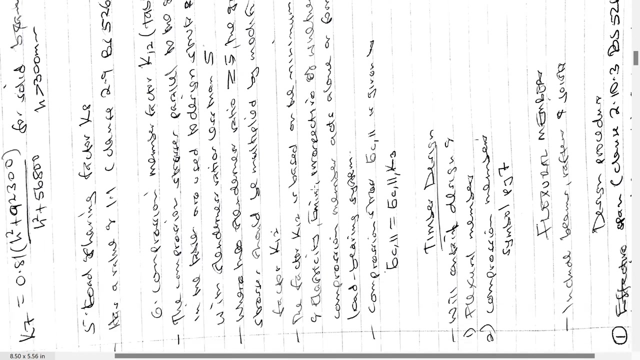 So it means when I'm calculating K12, I use E minimum, meaning E small value, not E mean average. I use E, this one here. I use E minimum irrespective of whether the load load compression member acts alone or forms part of the load sharing system. 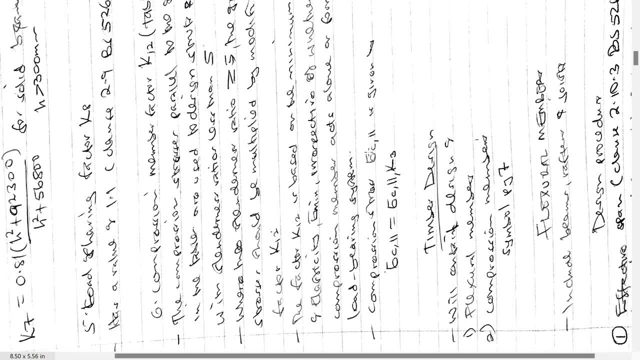 So you find that compression stress- this means compression stress, C means compression parallel- is given by compression stress. parallel is equal to compression stress multiplied by K3, which is load duration factor. So let's look at timber design. So in this particular course we look at two timber design related. 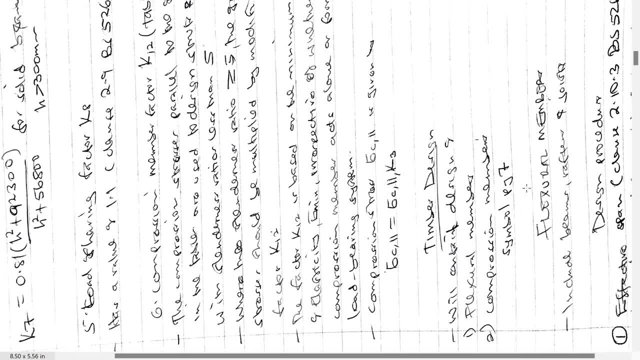 Okay, Design of flexural members, which include beams and slabs, Then design of compression members, which we said includes tracks and columns. So, if you want, we have a simple to show what is gross sectional area, what is breadth, what is depth, what is whatever of a timber section. 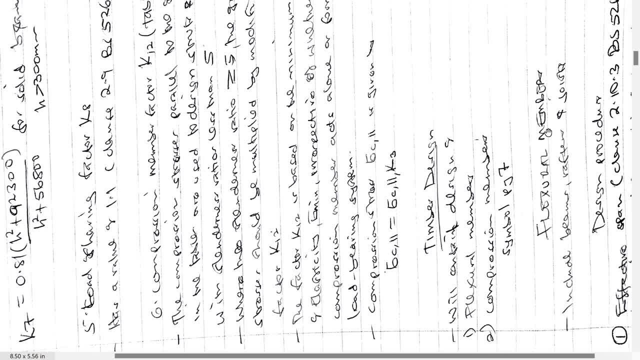 So let's look at flexural members. You see, include beams, rafters and joist. remember b, we know beams- uh, these are horizontal members. we know rafters are slanting members inclined daily. joists are maybe secondary beams, beams which transfer node to other beams. 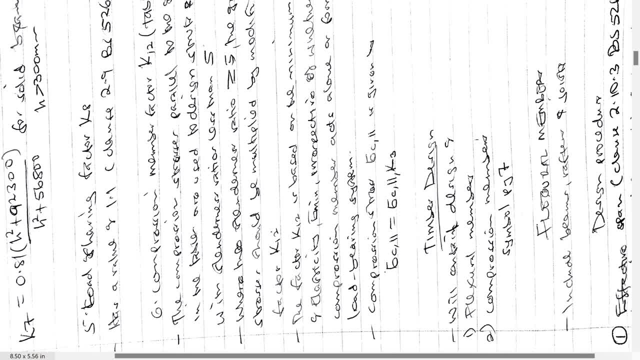 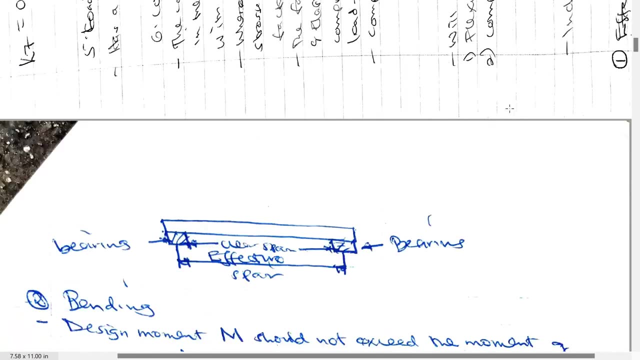 we have design procedure now for you to design this flexural member. step number one: you determine the effective span. effective span of the member which is given in clause 2, 10, 3 of bs 52, 68. so after effective span. now see the diagram here. now, from the diagram, we have what you call. 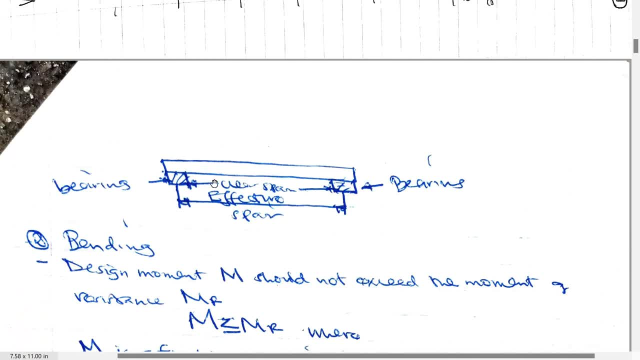 the bearings, two bearing on either side, we have what you call clear span, now effective span in the distance between the centers of the bearings, or some books will say distance between centers of support. so if you say this m2 center of support or center bearing, it will be right to mean the 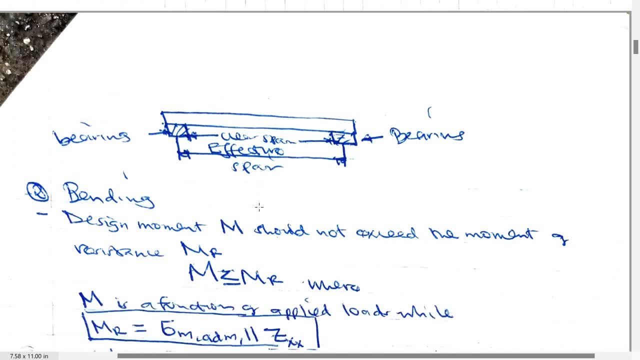 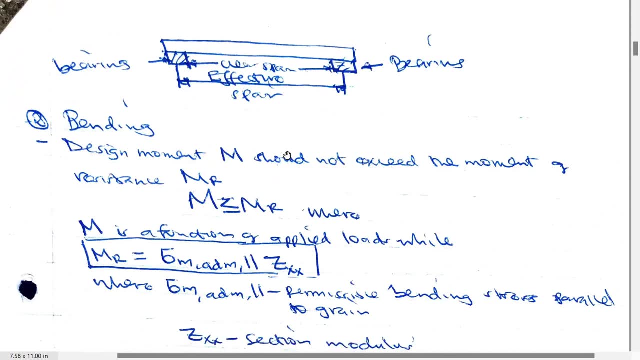 effective span, then now we have bending, now, after effective span, we go to bending now. in bending, remember, we have design moment and what we call moment of resistance. moment of resistance m? r is also called moment capacity. so in design moment capital m, it means moment which comes from the 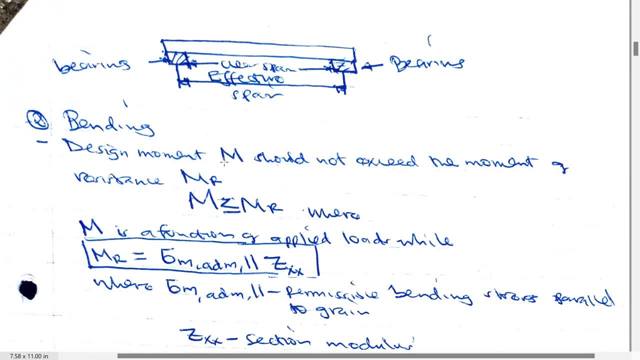 external loads being present applied to the timber section. but moment of resistance or moment capacity means the internal capability of that timber section to overcome the load being applied. so when you are designing the design moment, moment from load should be less or at once equal to the moment capacity or moment. 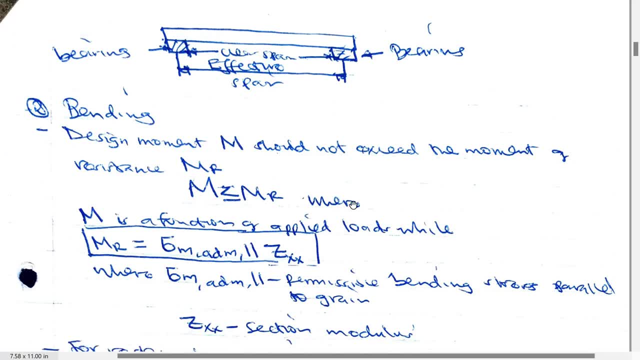 of resistance of this particular timber section. so where m design moment is a function of applied loads, while moment of resistance is a function of the internal capability of the timber section, which is given by permissible bending moment parallel to the grain multiplied by the section modulus along the x axis, which means z, x, x. so for rectangular section, 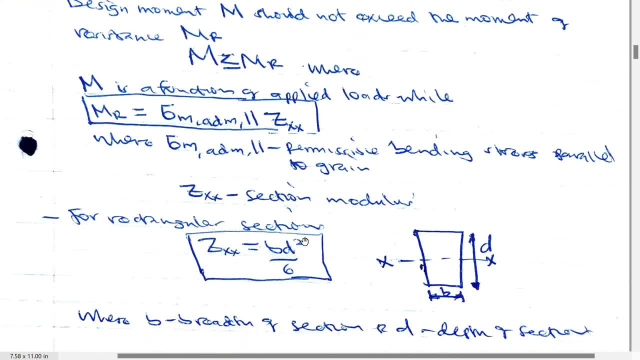 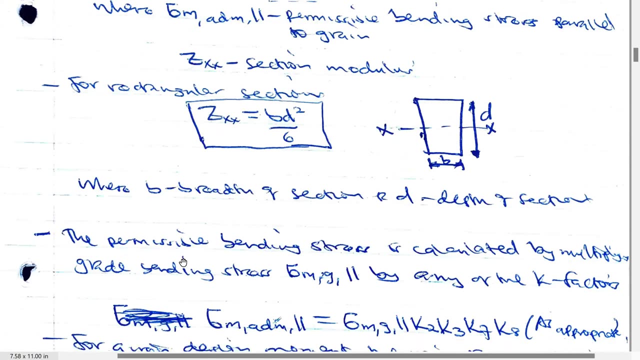 remember. But ZXX is given by BD squared over 6.. Now from the diagram here, D means depth, B means breadth. then along the XX axis. So the permissible bending stress is calculated by multiplying grade bending stress. Now, grade bending stress. this is what you obtain from the table. 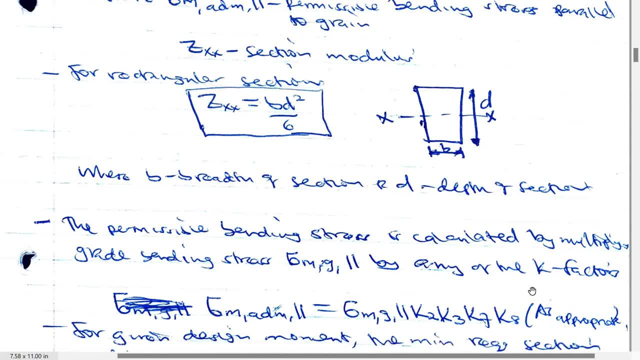 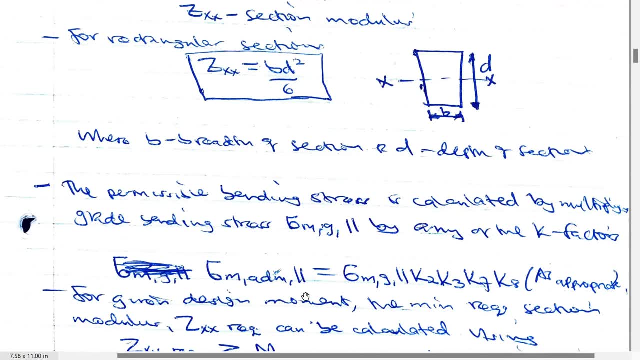 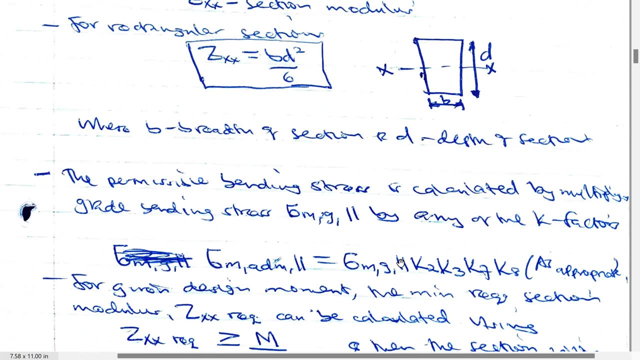 So you multiply by any of the K factors, which is appropriate, So permissible. now, when you see the word ABM, it means it is permissible. bending- So this one stands for parallel- is equivalent to bending stress. parallel to the grade obtained from the table multiplied by K2, by K3, by K7, by K8, as appropriate. 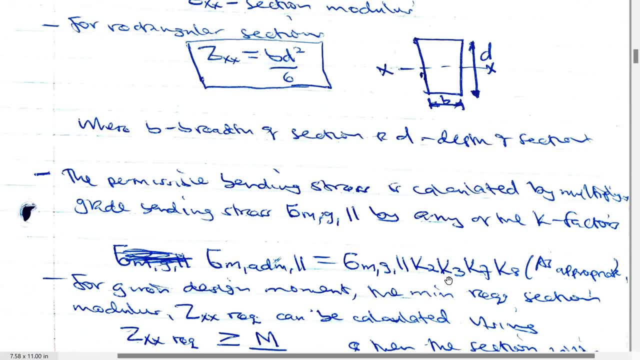 It means as appropriate means, maybe I only multiply by K3 and K8, or maybe by K3 and K7. It doesn't mean like we don't have, We don't have to include all the Ks in our calculation, depending on the equation. 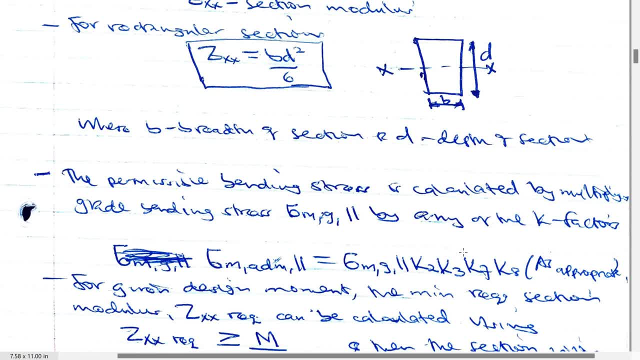 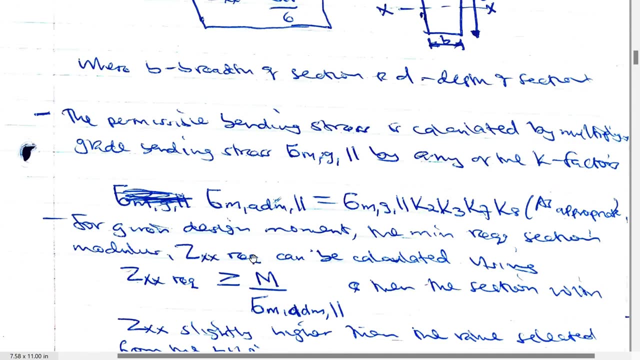 depending on the situation, we might take K2 and maybe K3, or we take K3 and K7. We don't have to put all of them in the same equation. So now, for a given design moment, the minimum required section modulus ZXX can be calculated using: 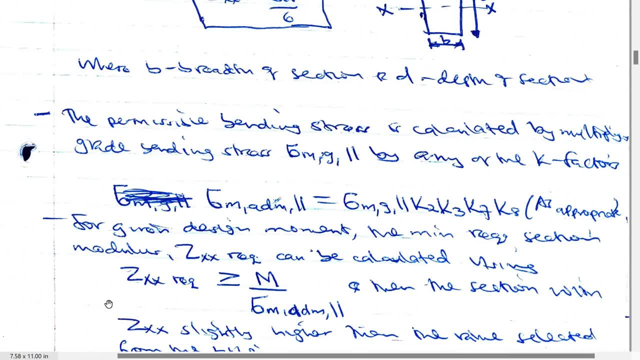 Now, remember we said that moment of resistance is equivalent to Permissible bending multiplied by section modulus Now, which should be greater or equal to design moment, which is M. So for me to find the minimum required ZXX, basically just divide by sigma M, ADM, parallel to both sides. 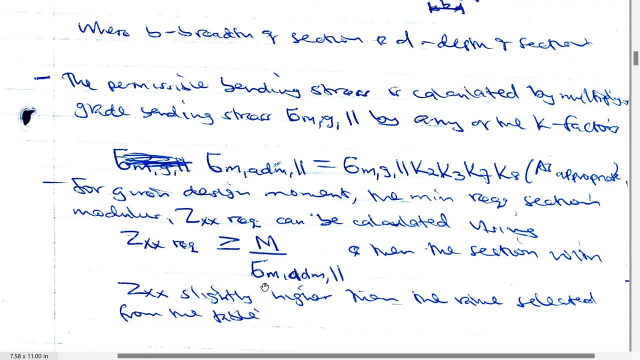 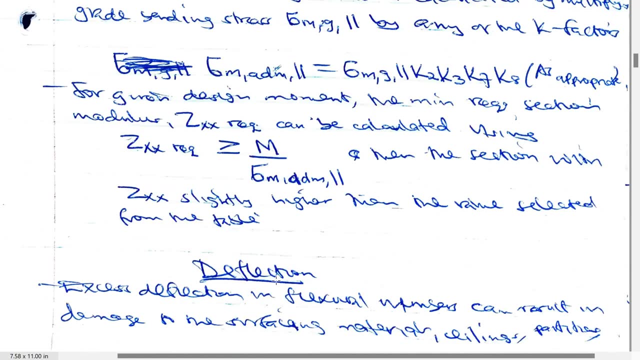 So that now, now, after I calculate this ZZ required, I will go to the table and obtain a section whose ZXX is equal to the minimum required. ZXX Section modulus along X. X is slightly greater than what I have calculated, So we go to deflection. 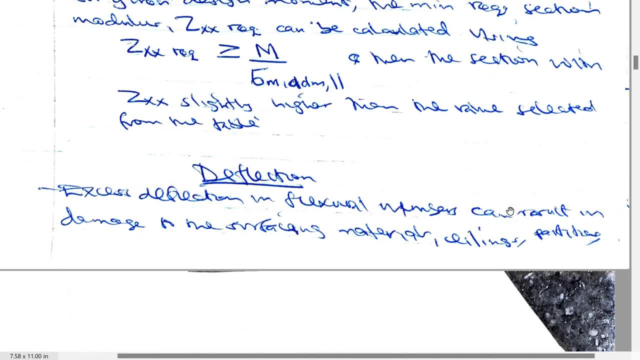 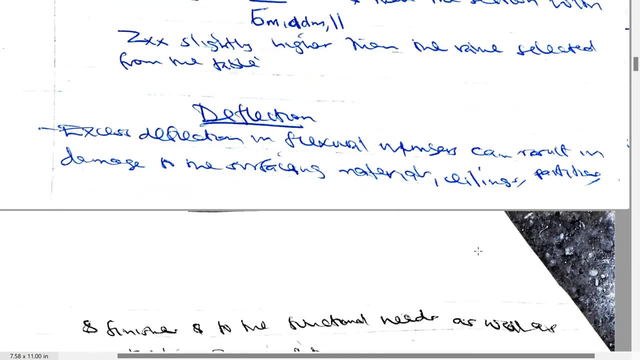 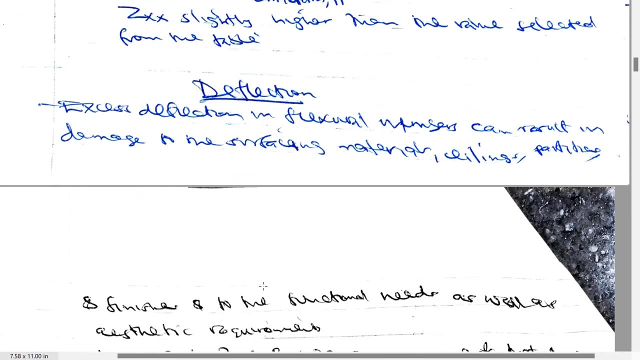 So excess deflection in flexural members can result in damage to the surfacing material, sailing partition and finishes and to the functional needs as well as aesthetic requirements. So when we maybe beam a flexural member undergoes Excessive deflection, you find that the surfacing material will be damaged. 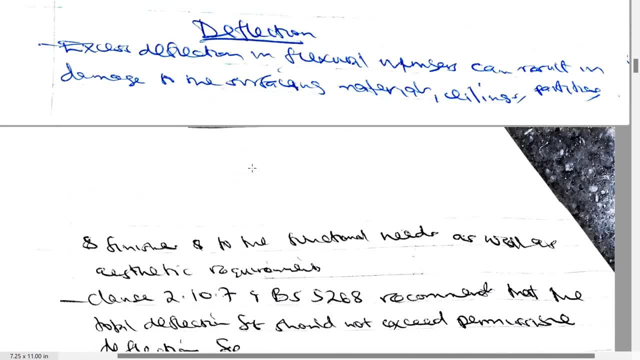 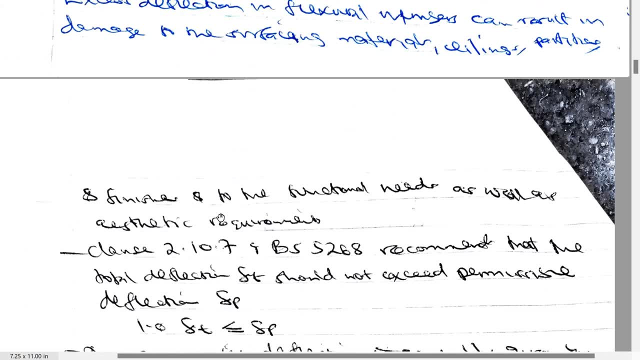 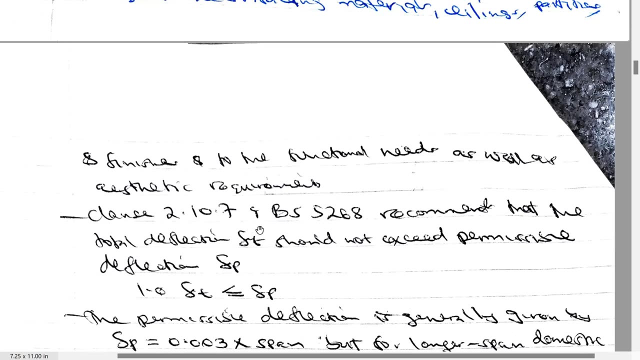 Even the ceiling will be damaged, even the partition and aesthetic value will remain like the shape of the house. It will appear sagging, which is not right. So clause 2107 of BS 5268 recommend that the total deflection, which is delta T, should not exceed permissible deflection delta P. 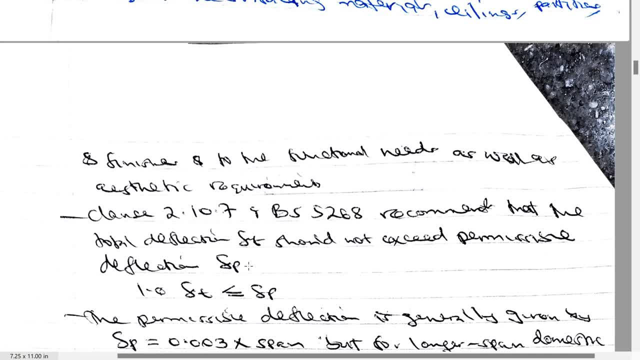 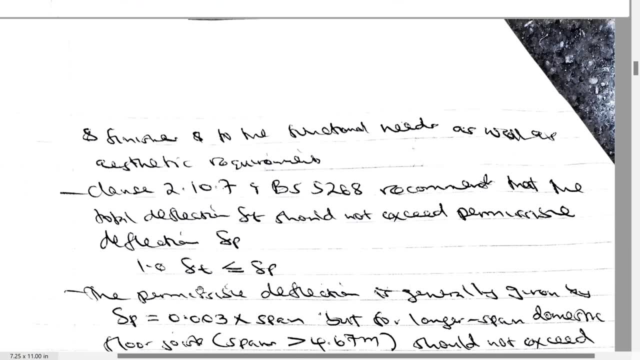 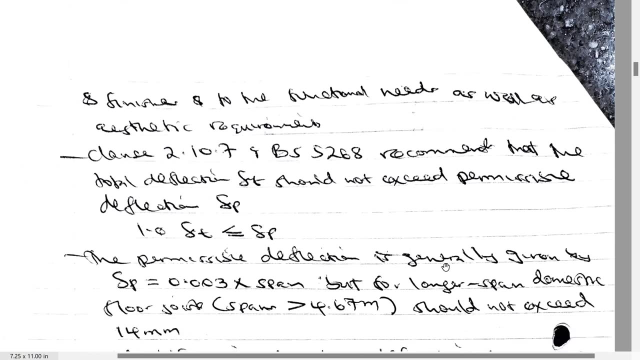 Now the total deflection. The total deflection should not be more than what is permitted, more than permissible. So in terms of equation I mean delta T should be less or equal to delta P. So the permissible deflection is generally given by: 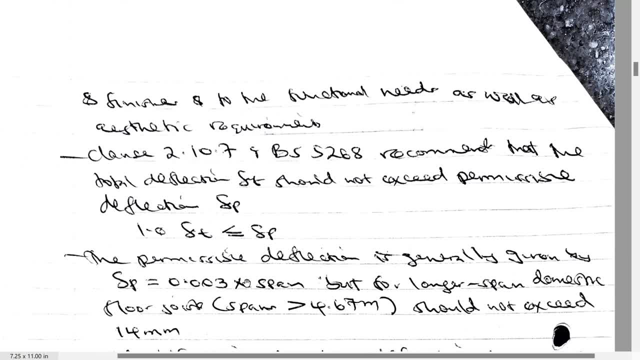 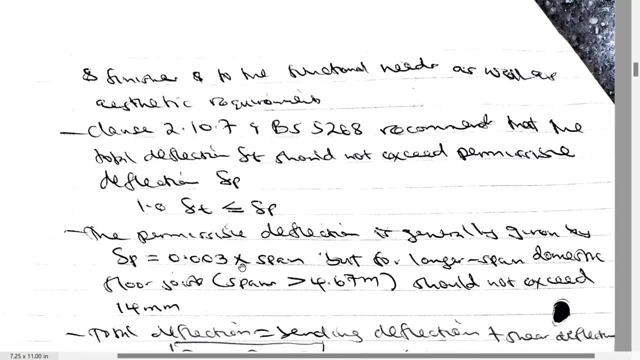 So permissible. delta P is equal to 0.003 times the effective span, But for longer span domestic flow is: If now your spans are more than 4.2,, more than 4.67 meters, you now restrict it to a maximum of 14 millimeters. 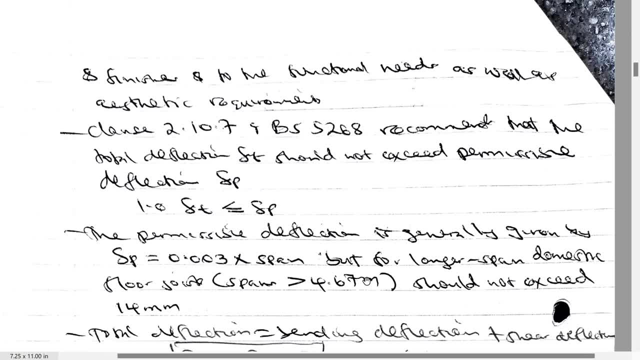 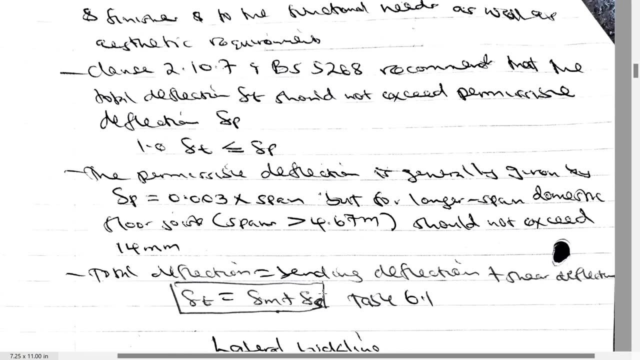 You don't use this formula If the span is more than 4.67, now your permissible should be 14 millimeters and not 0.003 times the span, So total deflection. Remember deflection comes from bending and shear force. 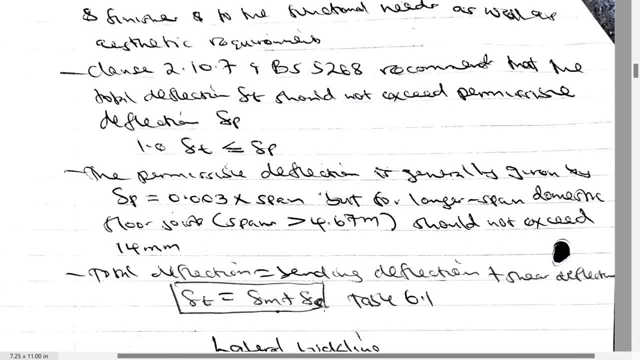 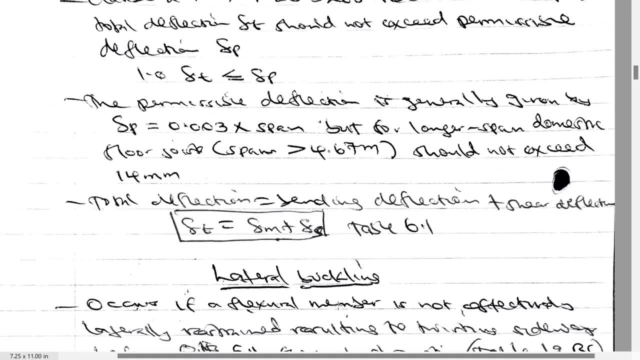 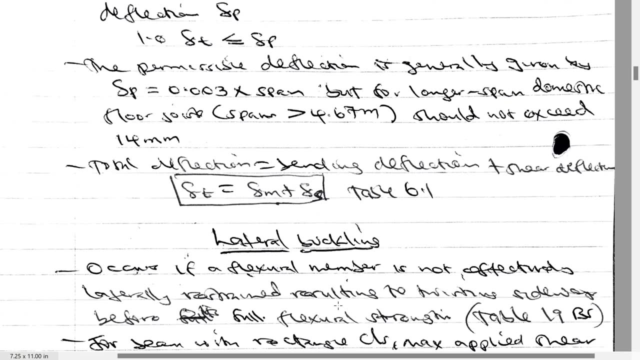 So you see that total deflection is equivalent to Is equivalent to bending Deflection plus shear deflection. Then we go to another thing, another test. we call lateral buckling. So lateral buckling, basically it means the timber section undergoes twisting. 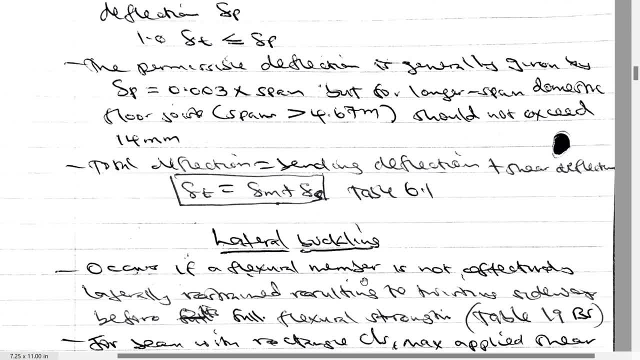 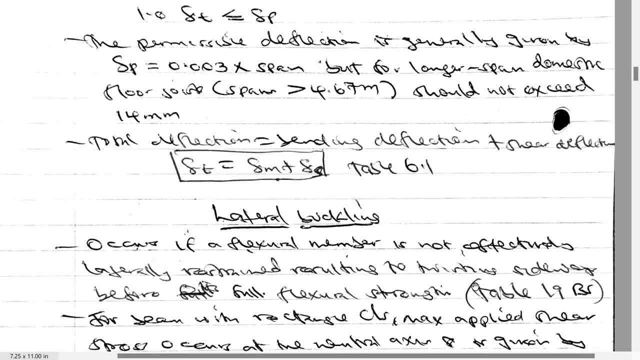 So we say occurs if a flexural member is not effectively laterally restrained, resulting to twisting sideways before its full flexural strength. Now it means lateral Lateral buckling is a mode of failure which occurs if the member is not restrained from rotation and lateral motion. 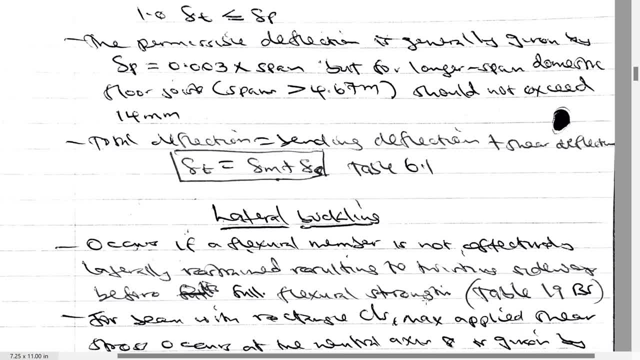 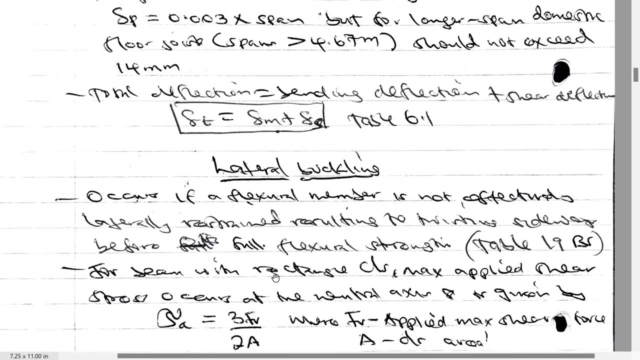 So by not being fully restrained you find like it will undergo twisting, and twisting is failure. So it's in table 19 of BS 5268.. It demonstrates what is a lateral buckling. So for beam with a rectangular Cross section. 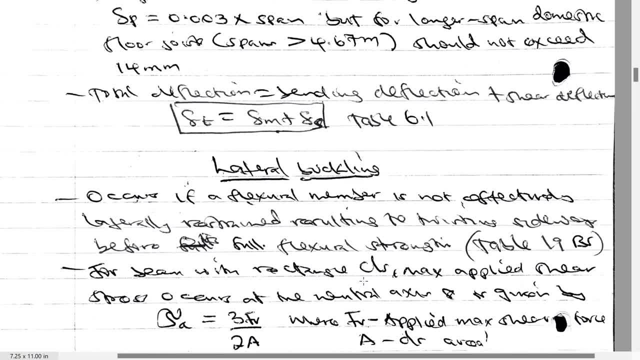 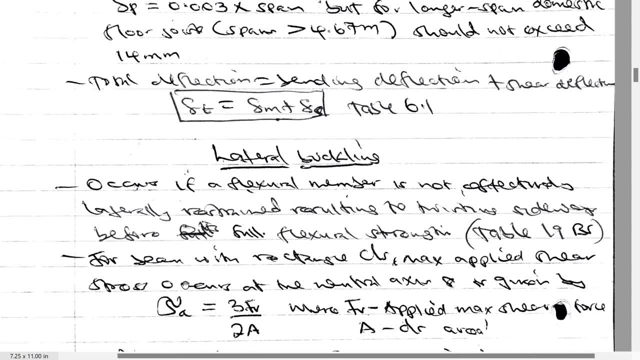 Now the most shape we use in timber section is a rectangular section. The maximum applied shear stress occurs at the neutral axis and is given by Now. the maximum applied- Now remember this- A stands for applied. Then shear stress applied is 3 times maximum shear force. FB divided by 2 times area. 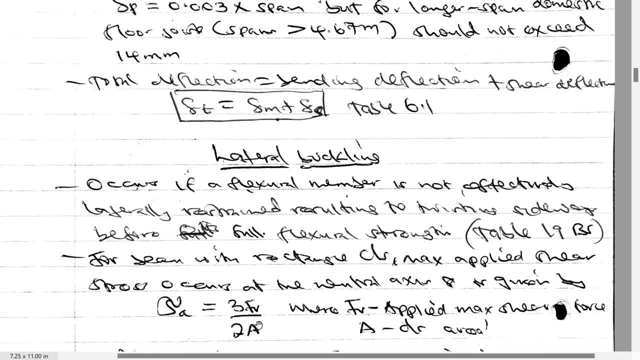 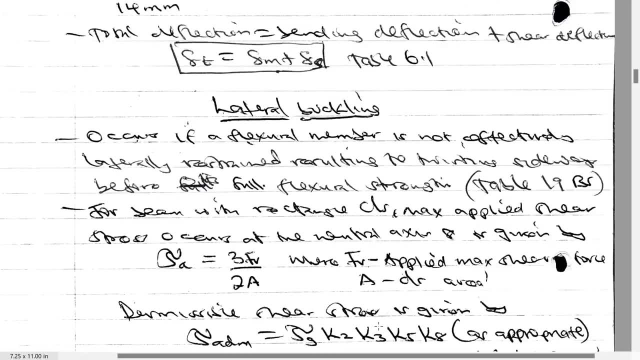 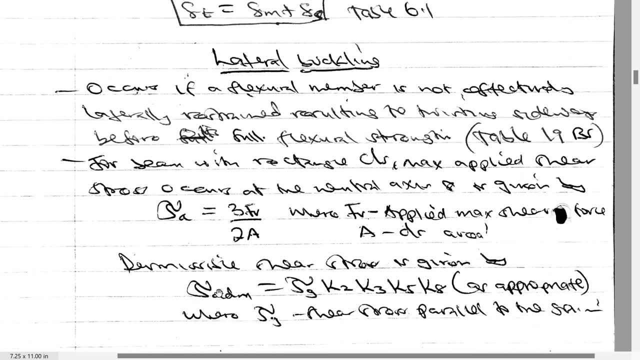 Now remember this area is obtained from the table along that timber section. So where FB is applied maximum shear force and A is cross-sectional area. So permissible shear stress is given by Now. permissible shear stress, Remember we said wherever we have ADM it means permissible. 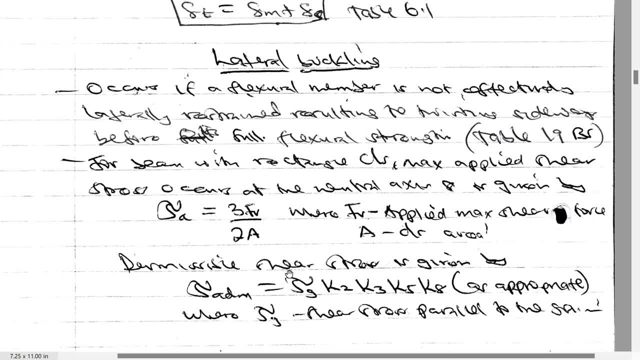 So it's given by shear stress obtained from the table multiplied by K2, K3, K5 or K8.. Like as appropriate means, It will depend on our equation. which K do we adopt? okay, So where sigma G, shear G means shear stress parallel to the grain. 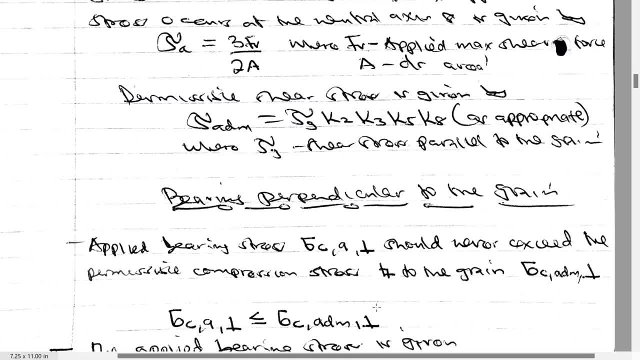 Then we go to bearing perpendicular to the grain. So we say applied bearing stress perpendicular to the grain should never exceed the permissible compression stress perpendicular to the grain. Now, applied is permissible. use ADM here because we say applied come from external load, while permissible come from the internal capability of our section. 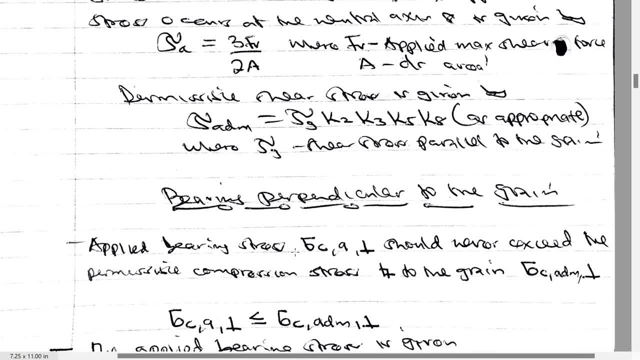 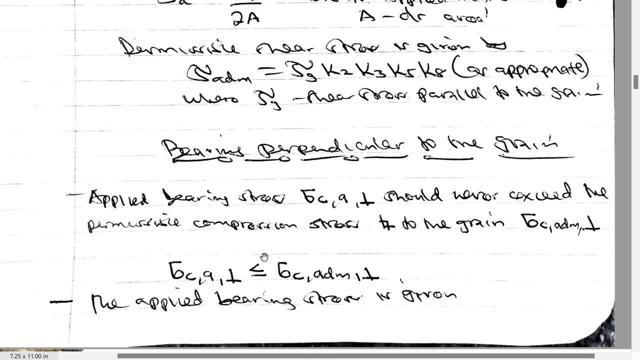 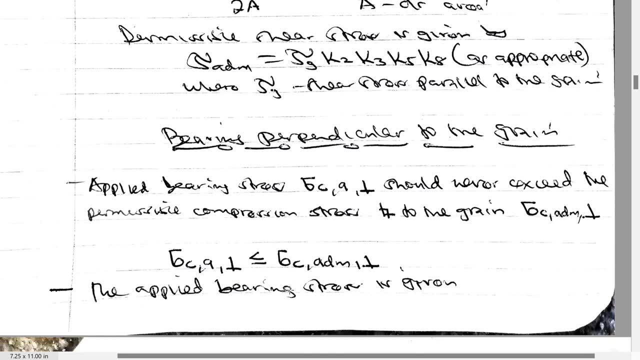 So for a section not to fail, it means applied should be less than what our section can carry. So this is the mathematical expression of applied: being less or at worst equal to the permissible. So the applied bearing. So applied bearing stress is given by 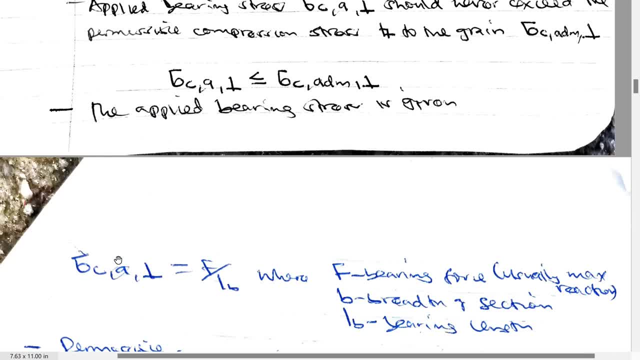 Now applied bearing stress is given by applied, which is sigma CA perpendicular, So it is bearing force F which is maximum reaction divided by- I'm sorry, we have B here- breadth of section multiplied by L subscript. B means bearing length, So this B here is missing. I'm sorry, students. 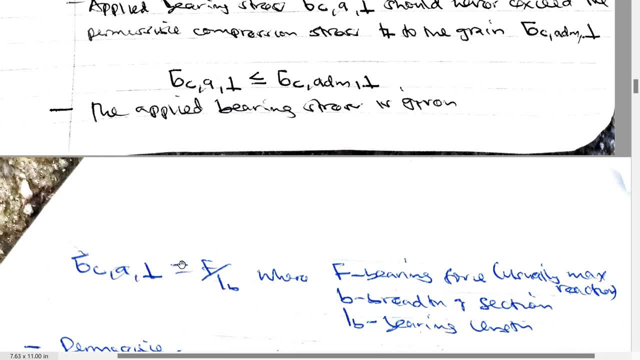 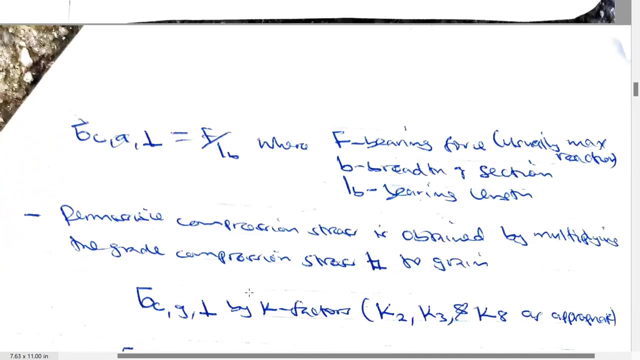 So ensure you add this B to be F, Because now Remember this bearing is stress. here stress is force over area. So if I have force here then I must divide by area. Area should be B multiplied by L, B. So permissible compression stress is obtained by multiplying the grade compression stress perpendicular to the grain. 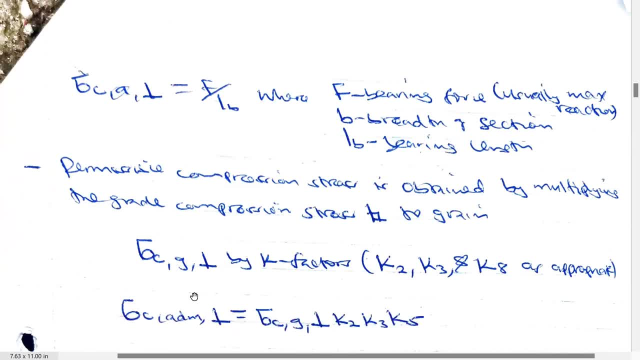 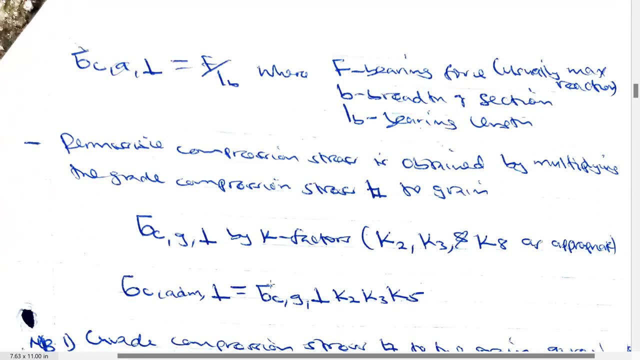 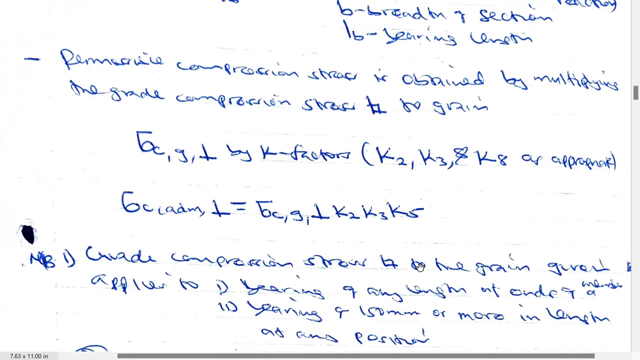 So if I want to give the permissible compression stress, which is that ADM, just multiply by this one obtained from the table, multiply by K2, multiply by K3 and multiply by K5.. So then now note the following grade compression stress perpendicular to the grain given applies to bearing of any length at the end of the member, bearing of 150 millimeter or more in length at any position.